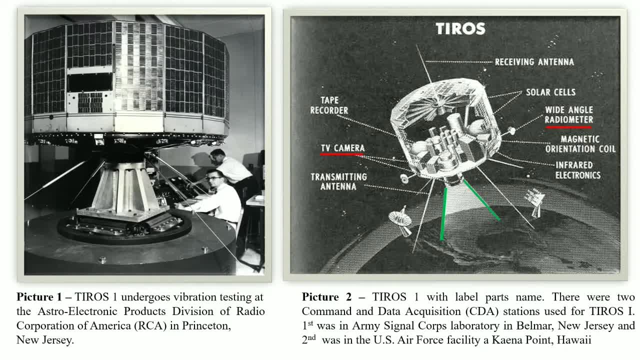 due to an electrical failure. during the 77 days it operated, the satellite sent back 19 389 usable pictures that we used in weather operations. tyros second was launched on november 23 1960. the first television picture sent from space by tyros one showed the new england coast and 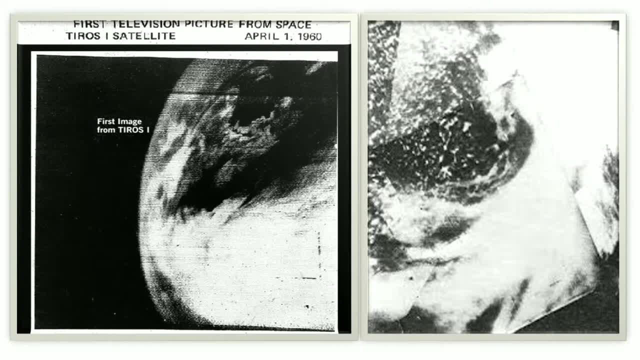 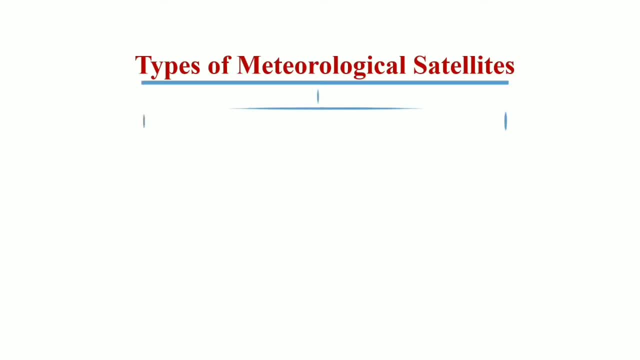 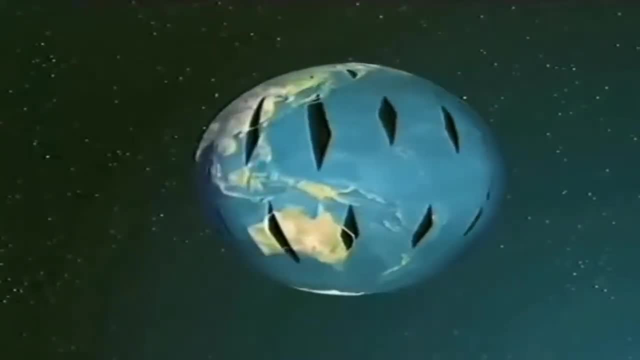 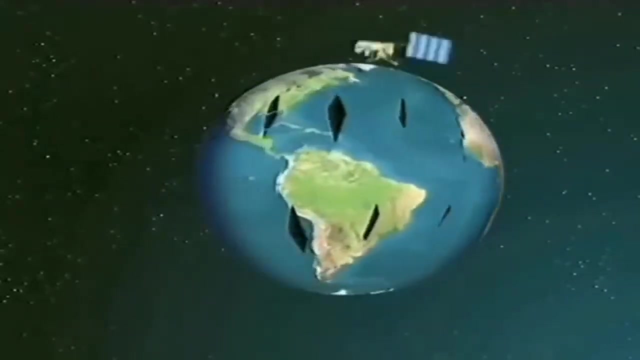 canada's maritime provinces north to the street lawrence river. basically meteorological satellite, classified into two types. the first one is polar orbiting satellite. polar orbiting satellites pass approximately over the poles at a height of about 850 kilometers. these satellites complete 14 orbits per day, so it can provide global coverage twice in 24 hours. 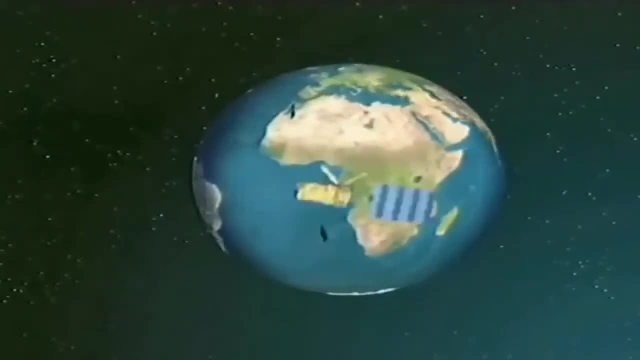 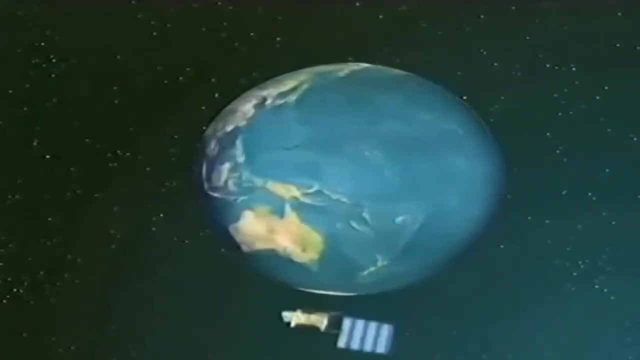 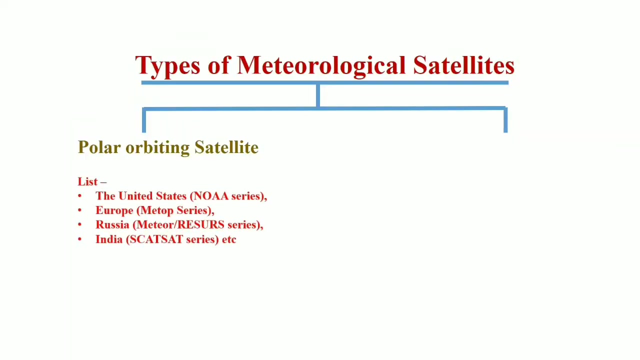 the area is scanned on each pass that is swath, usually about 2 600 kilometers wide. they provide meteorological data with better spatial resolution. the list of the some polar orbiting satellite name as per countries. now the second meteorological satellite name is geostationary orbiting satellite. 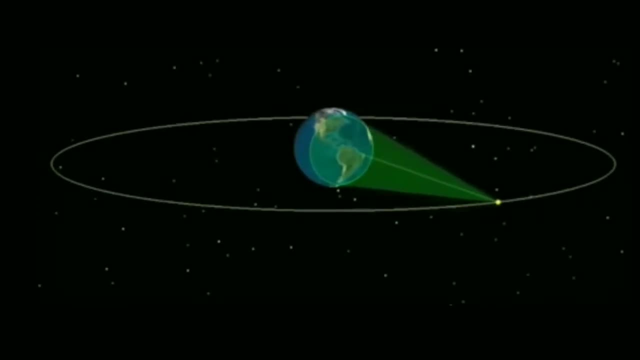 geostationary satellites orbit around the earth, over the equator, at a height of about 36 000 kilometers. they complete one orbit in 24 hours, synchronized with earth's rotation about its own axis. thus they remain over the same location, on the equator. 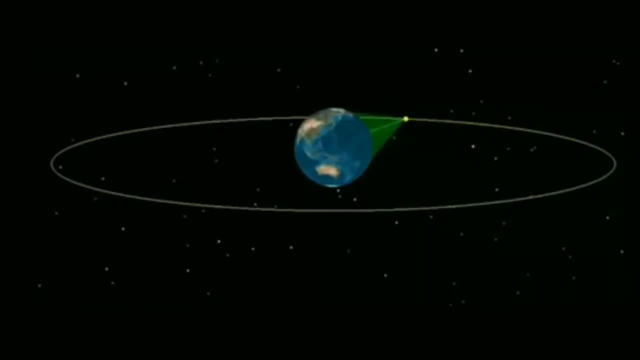 the main advantage of geostationary satellites lies in the high time scale resolution of their data. a fresh image of the full earth's disk is available every 30 minutes. however, they have limited spatial resolution as compared to the polar orbiting satellites. in view of their 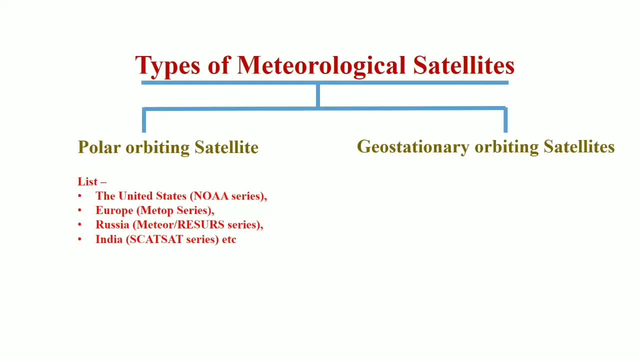 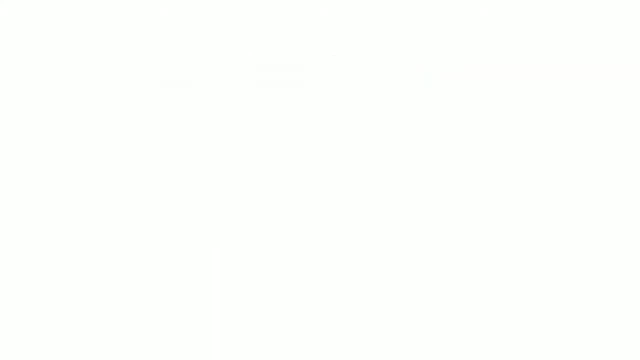 distance from the earth. some of the geostationary satellite listed below: india's first meteorological satellite, named metsat-1, which renamed as calpona 1, launched in september 12 2002, which entered geostationary orbit. it carry very high resolution radiometer capable of imaging the earth in the visible 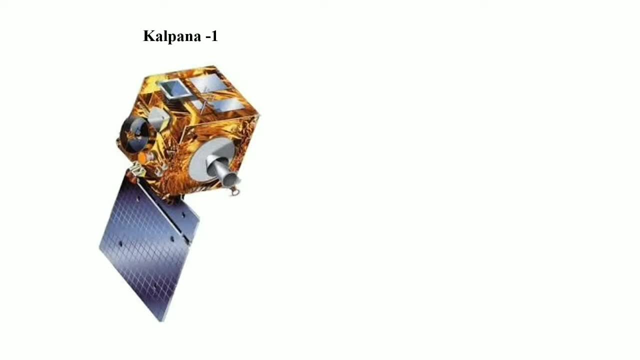 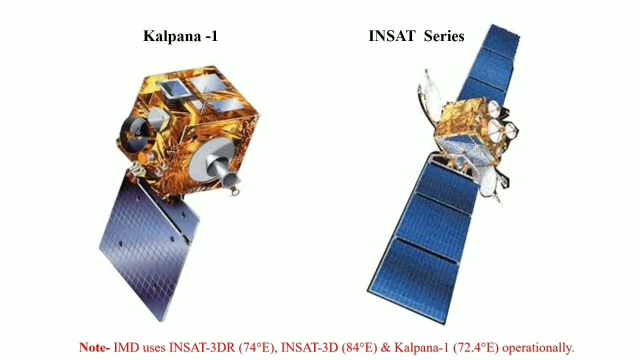 thermal, infrared and water vapor bands. after that, the indian national satellite. inside is a multi-purpose geostationary satellite which carries both meteorological and communications payloads. the very high resolution radiometer scans are every three hours on routine basis, and half hourly to even less than that for 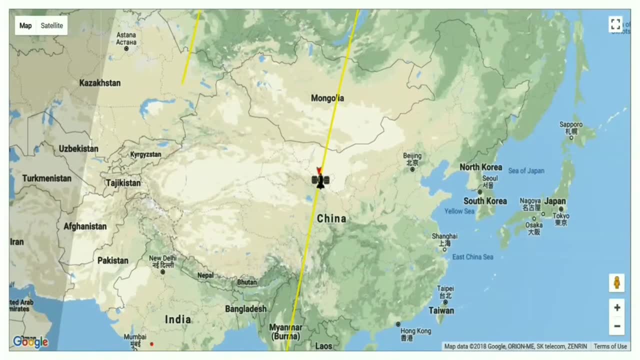 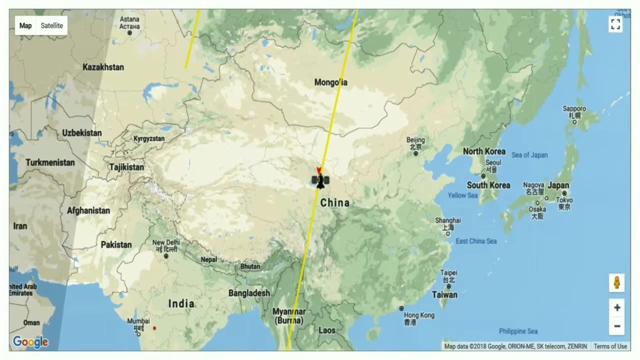 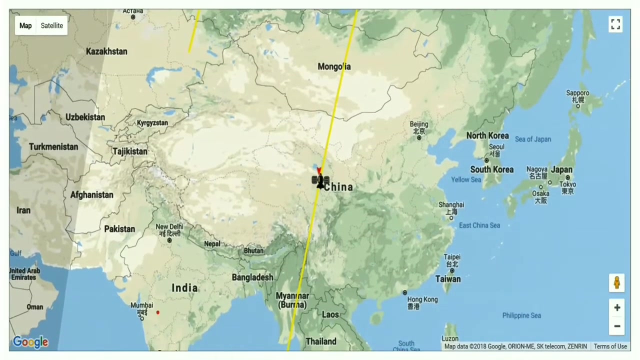 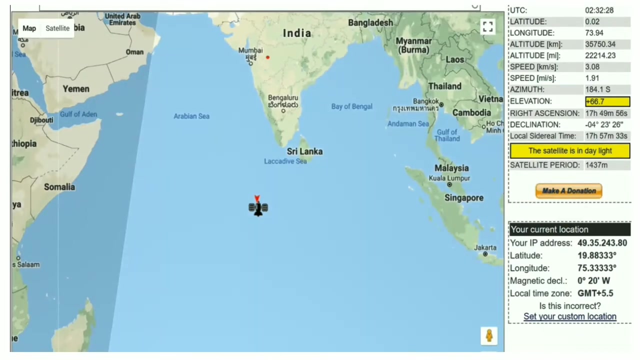 monitoring cyclones, etc. here we see that the track of weather forecasting polar orbiting satellite of India, scat, sat 1 over the altitude 724 kilometers from ground and satellite period is 99.3 minutes. similarly, we could see that the weather forecasting geostationary satellite of India inside 3d are over. 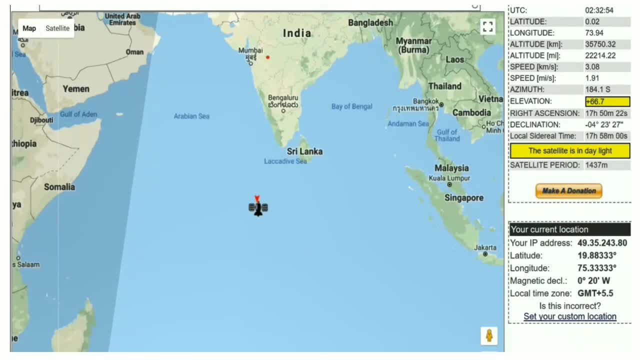 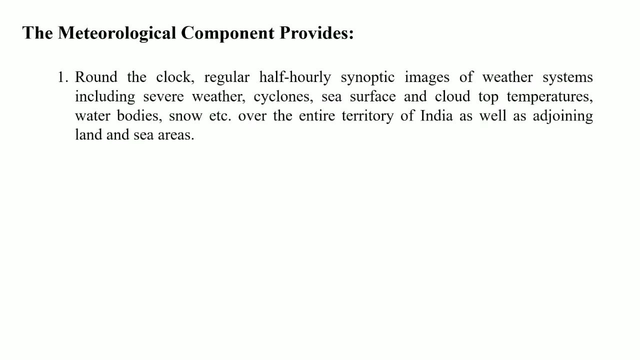 the altitude 35,000 750 kilometers from ground and satellite period is 1437 minute. the meteorological component provides round-the-clock, regular, half-hourly synoptic images of weather systems, including severe weather, cyclones, sea surface and cloud weather systems, including severe weather, cyclones, sea surface and cloud. 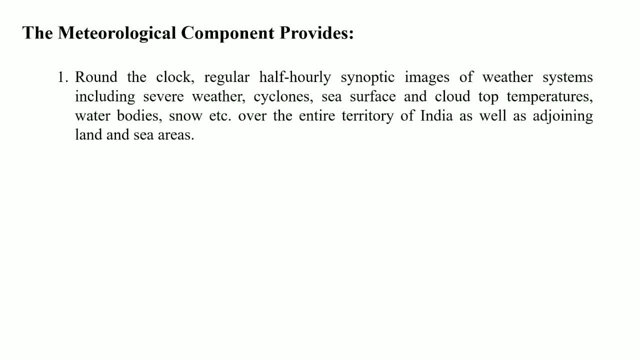 cyclones, sea surface and cloud. cyclones, sea surface and cloud, top temperatures, water bodies, snow, etc. over the entire territory of India. as top temperatures, water bodies, snow, etc. over the entire territory of India. as top temperatures, water bodies, snow, etc. over the entire territory of India, as well as adjoining land and sea area. 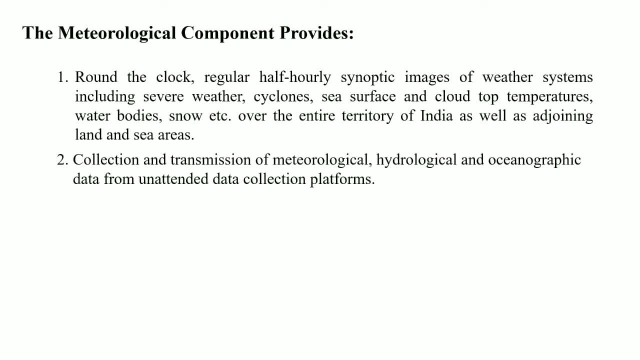 well as adjoining land and sea area, well as adjoining land and sea area. collection and transmission of collection and transmission of collection and transmission of meteorological, hydrological and meteorological, hydrological and meteorological, hydrological and oceanographic data from unattended data. oceanographic data from unattended data. 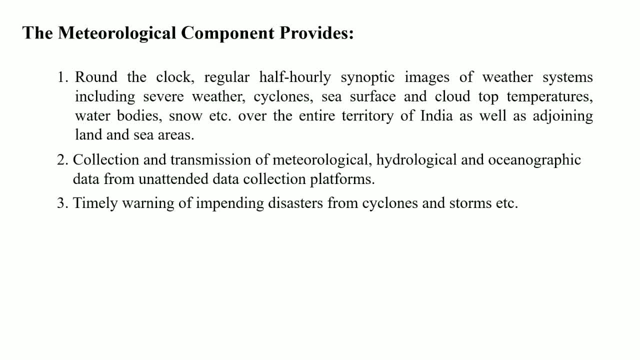 oceanographic data from unattended data collection platform: timely warning of collection platform. timely warning of collection platform. timely warning of impending disasters from cyclones and impending disasters from cyclones and impending disasters from cyclones and storms, etc. dissemination of meteorological storms, etc. dissemination of meteorological. 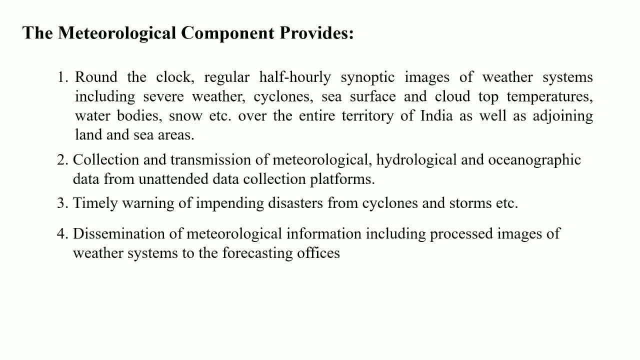 storms, etc. dissemination of meteorological information, including processed information, including processed information, including processed images of weather systems, to the images of weather systems, to the images of weather systems to the forecasting offices. satellite sensors for forecasting offices. satellite sensors for forecasting offices. satellite sensors for meteorological application, which. 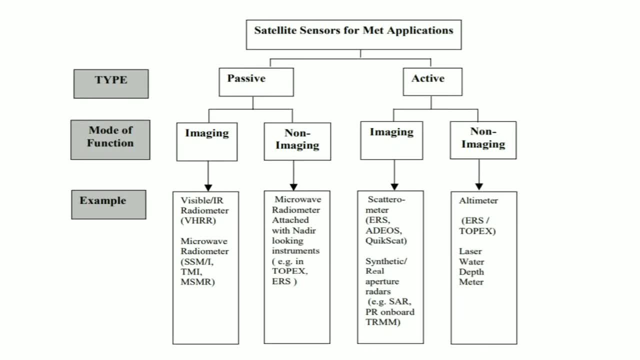 meteorological application, which meteorological application which further classified as passive and active, further classified as passive and active, further classified as passive and active sensor types, and that further sensor types and that further sensor types and that further sub classification is done by imaging and sub classification is done by imaging. and 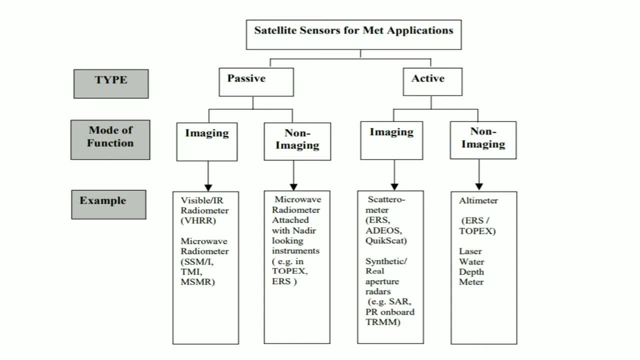 sub classification is done by imaging and non imaging sensor. here we see that non imaging sensor. here we see that non imaging sensor. here we see that the very high resolution radiometer is the very high resolution radiometer is the very high resolution radiometer, is under passive imaging type sensor, which 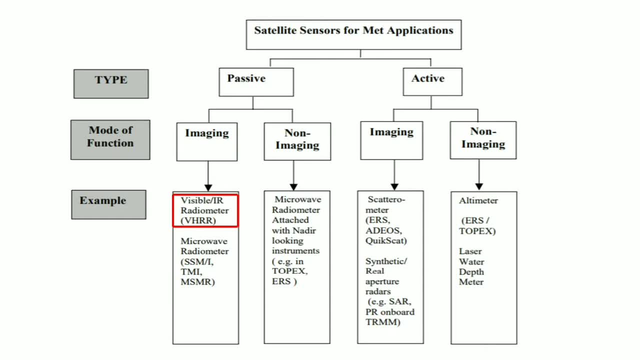 under passive imaging type sensor, which under passive imaging type sensor, which is developed in India by satellite, is developed in India by satellite, is developed in India by satellite application Center Ahmedabad, whereas the application Center Ahmedabad, whereas the application Center Ahmedabad, whereas the scatterometer is under the active types. 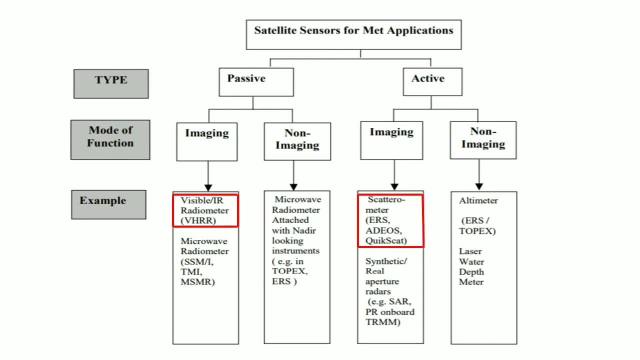 scatterometer is under the active types scatterometer is under the active types sensor and remaining one is under the sensor and remaining one is under the sensor and remaining one is under the passive- non imaging and active- non passive, non imaging and active- non passive, non imaging and active- non imaging sensors- the three most common. 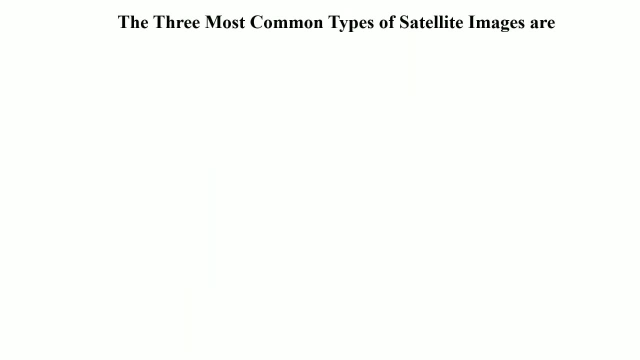 imaging sensors. the three most common imaging sensors, the three most common types of satellite images, which prefer types of satellite images, which prefer types of satellite images which prefer by scientists, are first one is visible by scientists. are first one is visible by scientists. are first one is visible satellite image. second one is infrared. 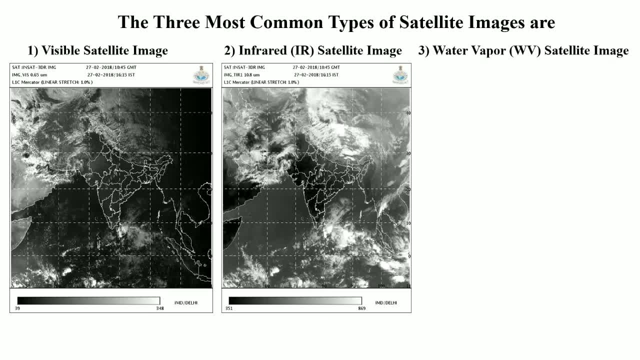 satellite image. second one is infrared satellite image. second one is infrared satellite image. and third one is water satellite image. and third one is water satellite image and third one is water vapor satellite image. these different vapor satellite image, these different vapor satellite image, these different images refer to what part of the 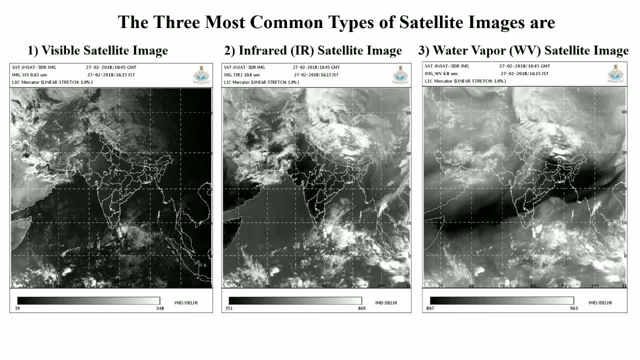 images refer to? what part of the images refer to what part of the electromagnetic spectrum? the satellite electromagnetic spectrum, the satellite electromagnetic spectrum. the satellite sensors are sampling these images took. sensors are sampling these images took. sensors are sampling these images took from inside 3d, our satellite. at same. 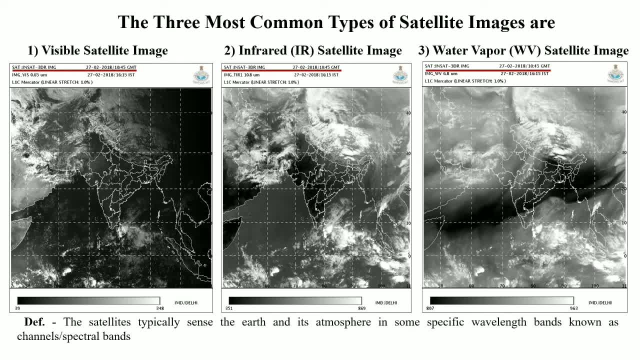 from inside 3d, our satellite, at same. from inside 3d, our satellite, at same time. for visible satellite images. time for visible satellite images. time for visible satellite images. atmospheric windows is 0.6 microns for atmospheric windows is 0.6 microns for. 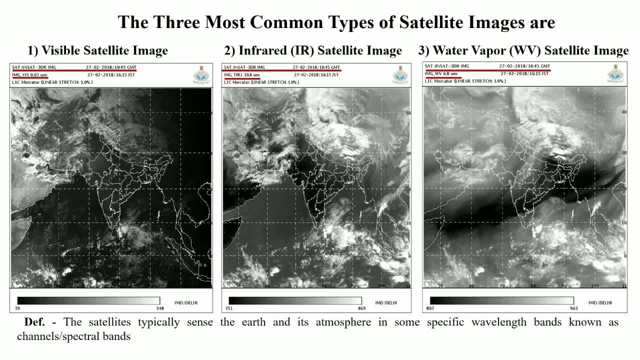 atmospheric windows is 0.6 microns. for infrared satellite images between 10 to infrared satellite images between 10 to infrared satellite images between 10 to 12 microns. and for the water vapor: 12 microns. and for the water vapor: 12 microns. and for the water vapor images, which includes radiation, 6.5 to. 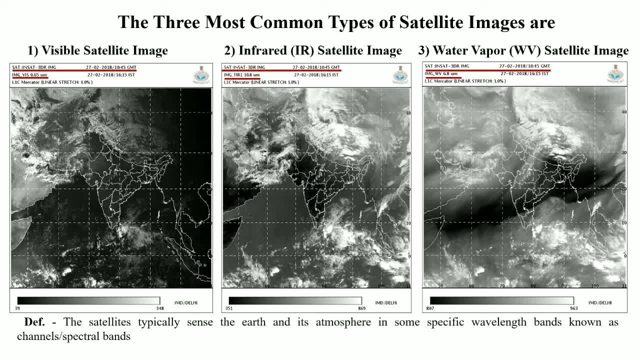 images which includes radiation 6.5 to. images which includes radiation 6.5 to 6.9 microns in the electromagnetic 6.9 microns in the electromagnetic 6.9 microns in the electromagnetic spectrum. these images are in marketer. 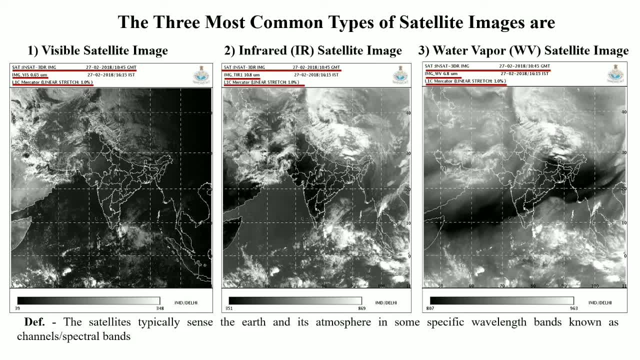 spectrum. these images are in marketer spectrum. these images are in marketer projection of linear stretch by 1%, but projection of linear stretch by 1%, but projection of linear stretch by 1%. but what is Mercator projection? let us see what is Mercator projection? let us see. 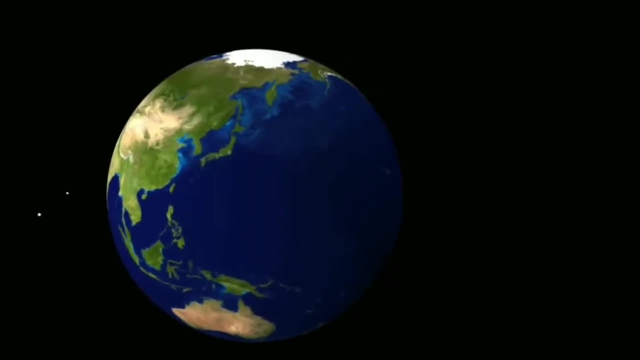 what is Mercator projection? let us see: Mercator projection is a tool that Mercator projection is a tool. that Mercator projection is a tool that transforms the Earth's surface into a, transforms the Earth's surface into a. transforms the Earth's surface into a flat plane that can be shown on paper or 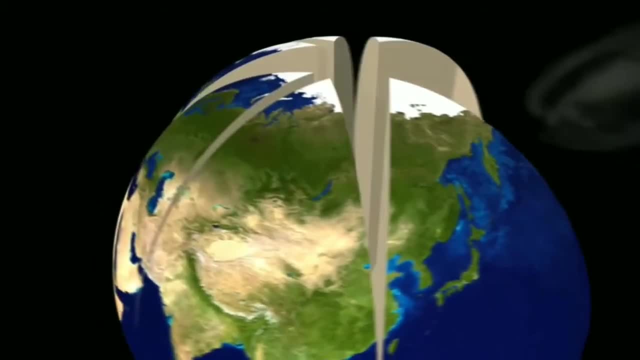 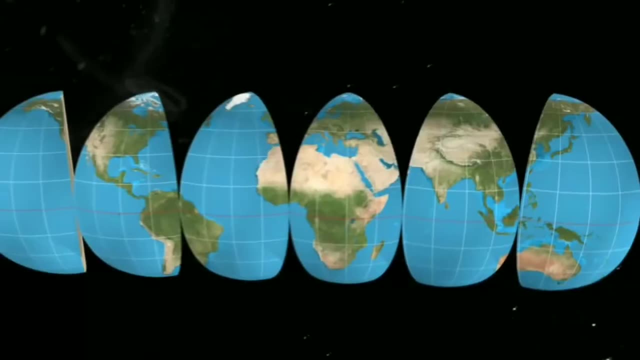 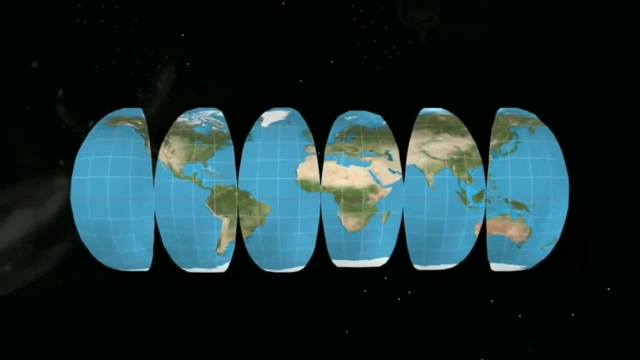 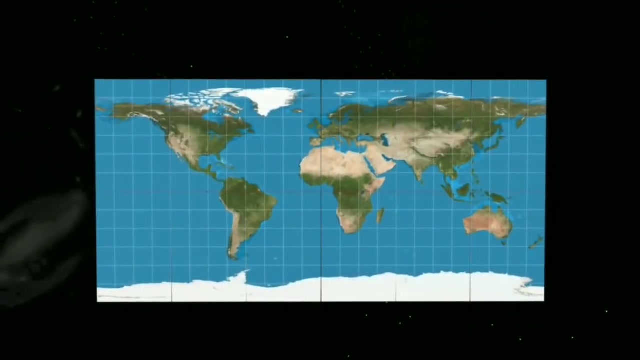 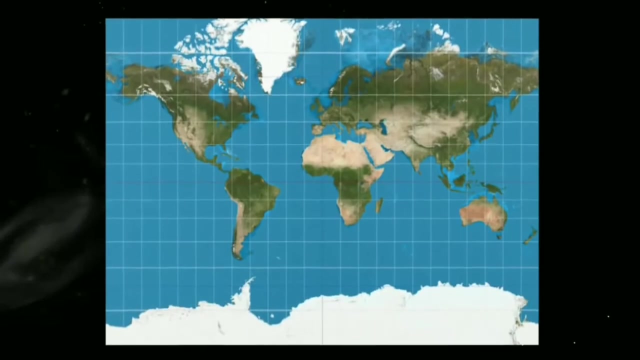 flat plane that can be shown on paper, or flat plane that can be shown on paper or digital maps, by stretching it with digital maps, by stretching it with digital maps, by stretching it with suitable linear percentage, suitable linear percentage, suitable linear percentage. now see some satellite view of cyclone. 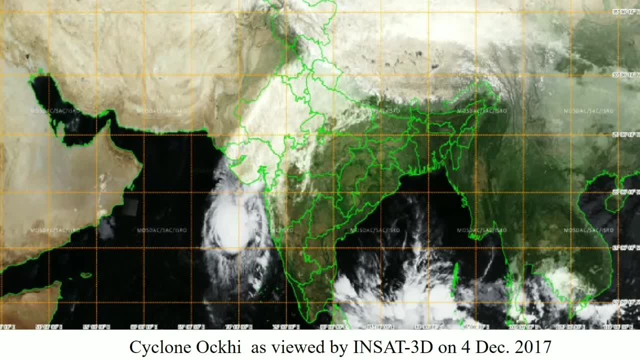 now see some satellite view of cyclone. now see some satellite view of cyclone over Indian region. this image show that over Indian region. this image show that over Indian region. this image show that very severe cyclonic storm Aki cyclone. very severe cyclonic storm Aki cyclone. very severe cyclonic storm Aki. cyclone Aki originated as a depression off Aki. originated as a depression off Aki originated as a depression off southeast coast of Sri Lanka, touched southeast coast of Sri Lanka, touched southeast coast of Sri Lanka, touched Kanyakumari and finally crossed. 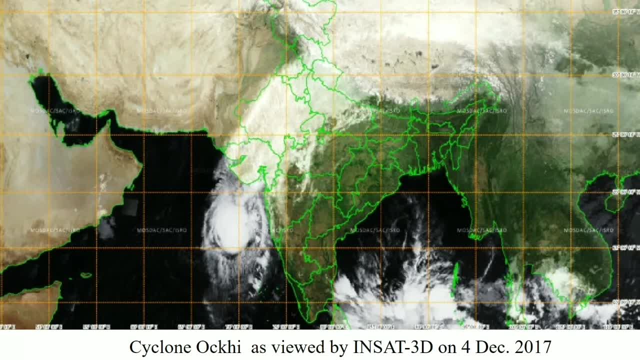 Kanyakumari and finally crossed Kanyakumari. and finally crossed gharat coast on December 5th 2017. many gharat coast on December 5th 2017. many gharat coast on December 5th 2017. many died and many fishermen from Tamil Nadu. 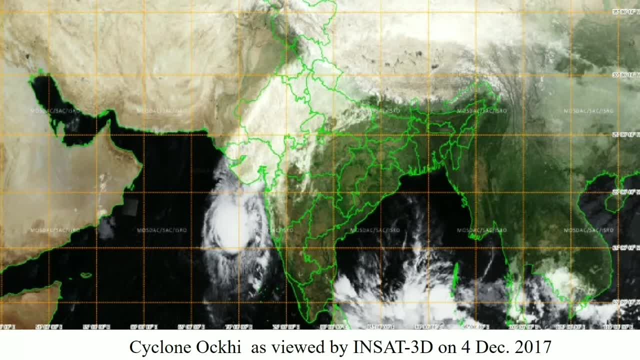 died and many fishermen from Tamil Nadu died and many fishermen from Tamil Nadu and Kerala could not be traced. it is one and Kerala could not be traced. it is one and Kerala could not be traced. it is one of the costliest cyclone in Indian Ocean. of the costliest cyclone in Indian Ocean. 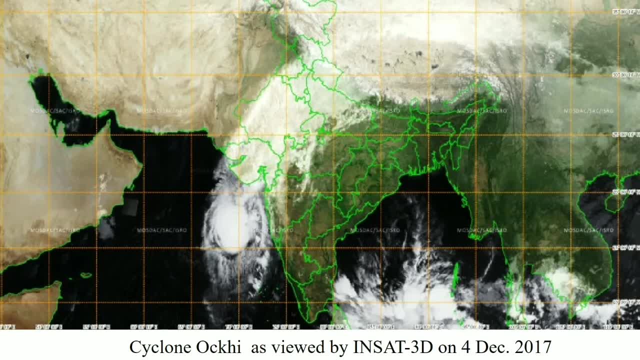 of the costliest cyclone in Indian Ocean in recent history. cyclone ro anew was a in recent history. cyclone ro anew was a in recent history. cyclone ro anew was a relatively weak tropical cyclone. that relatively weak tropical cyclone, that relatively weak tropical cyclone that caused severe flooding in Sri Lanka and 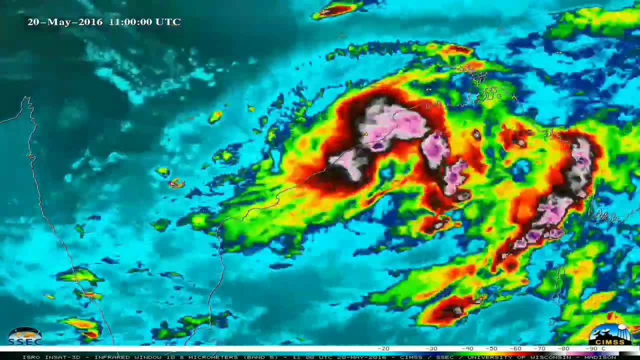 caused severe flooding in Sri Lanka and caused severe flooding in Sri Lanka and Bangladesh. it formed on 17 May and Bangladesh. it formed on 17 May and Bangladesh. it formed on 17 May and dissipated on 23rd of May 2016. it is the. 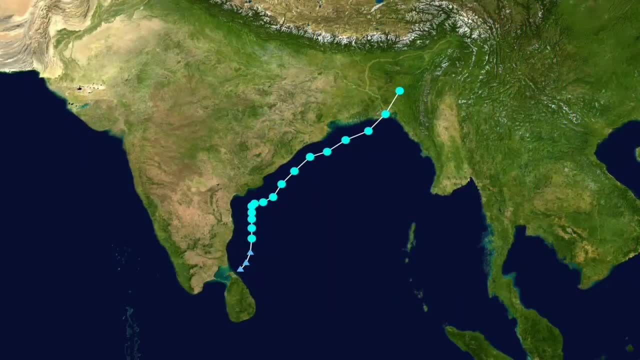 dissipated on 23rd of May 2016. it is the dissipated on 23rd of May 2016. it is the first tropical cyclone of the annual first tropical cyclone of the annual first tropical cyclone of the annual cyclone season: ro anew cyclone originated. cyclone season ro anew. cyclone originated. cyclone season ro anew. cyclone originated from a low-pressure area that formed from a low-pressure area that formed from a low-pressure area that formed south of Sri Lanka, which gradually south of Sri Lanka, which gradually south of Sri Lanka, which gradually drifted north and intensified into a 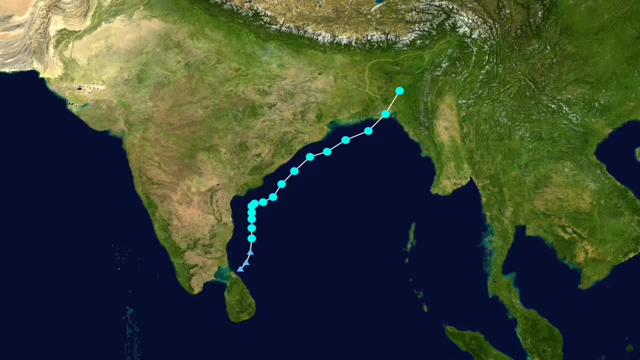 drifted north and intensified into a. drifted north and intensified into a cyclonic storm of 19 May. satellite cyclonic storm of 19 May. satellite cyclonic storm of 19 May. satellite imagery is an invaluable source of imagery is an invaluable source of imagery is an invaluable source of information for operational forecasters. 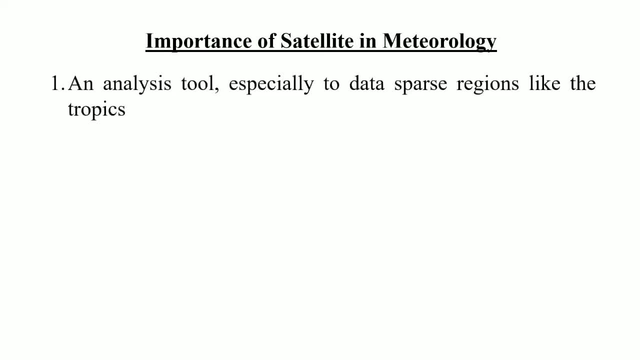 information for operational forecasters. information for operational forecasters. it is being used as first an analysis. it is being used as first an analysis. it is being used as first an analysis tool, especially to data sparse regions tool, especially to data sparse regions tool, especially to data sparse regions like the tropics. second, direct aid to